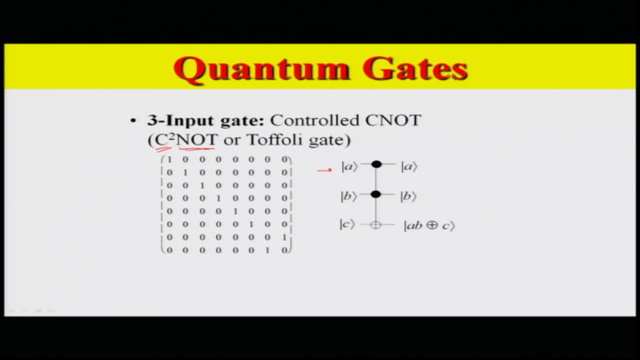 the bit flip. So A, B are the control bits and C is the one which undergoes the change, and this is more often also known as the Toffoli gate. The Toffoli gate is either known as CC, NOT gate, or the Toffoli gate and a typical matrix. 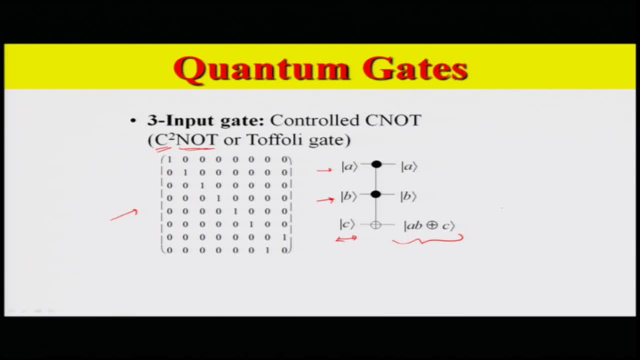 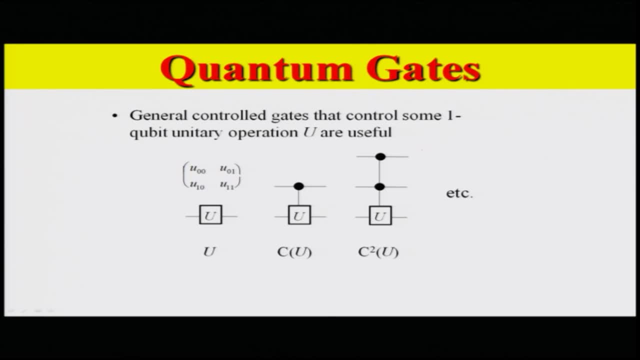 for such a gate is given by this for three qubits, A generalized control gate that can control some one qubit. unitary operation U are useful and that can be looked at in this format where every time you have an operation it is possible to control the control bit. 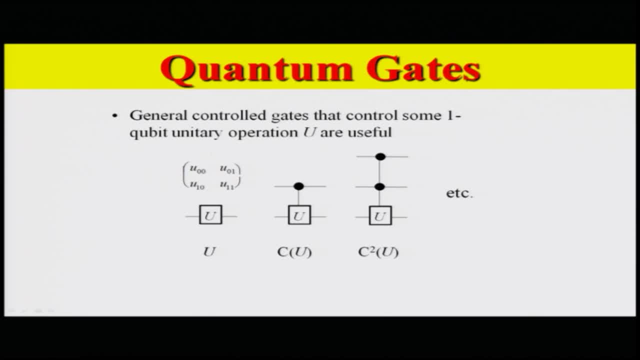 and the other one. So the control bits are placed in such a way that when the operation is going we can label them in terms of the operation. So, for example, just a unitary operation of the kind in circuit times would be looking like this, which we represent by U Once we use. 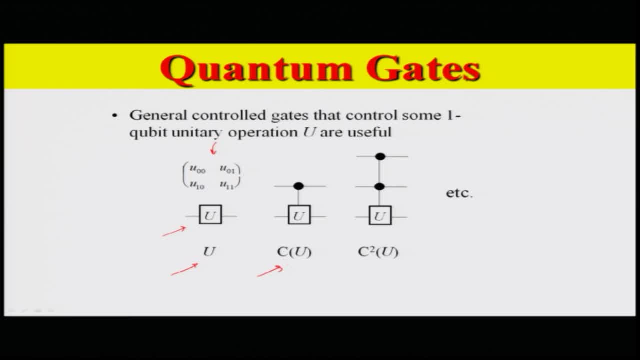 it with respect to a single control, then it is a control on top of the operation. So that is an example of the control NOT. So our unitary operation was essentially the NOT operation that we showed was unitary and that is the one which is being used in all. 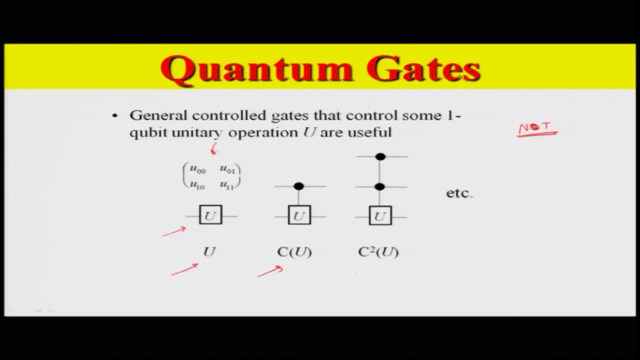 these cases here with some control. If we use two controls then it becomes control control unitary and this can be scaled, as we have seen, to further kind of processes where more and more control bits can be used. However, to have a universal gate we need 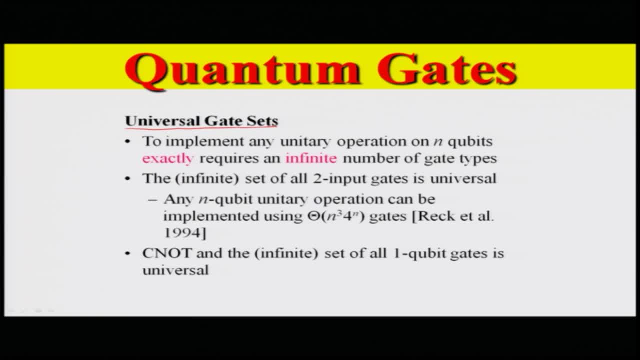 a gate set which will implement any unitary operation on N qubits exactly would require an infinite number of gate types. So the principle that we showed for a single qubit case where we were able to use only two gates as a complete set, the Hadamard and the phase. 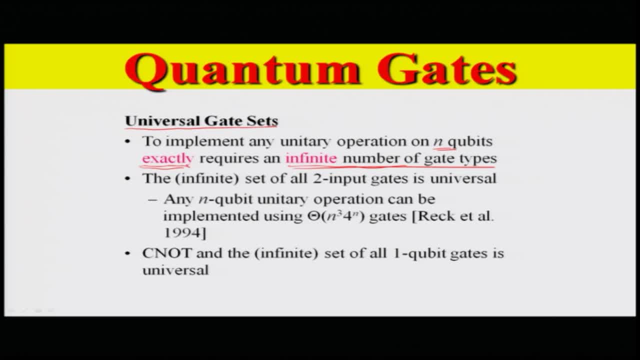 rotation not as simple as we go to higher number of qubits, and so the complete set gets harder and harder to be defined. The infinite set of all two input gates is universal, for instance, So any n qubit unitary operation can be implemented using so and so many gates, and this is sort 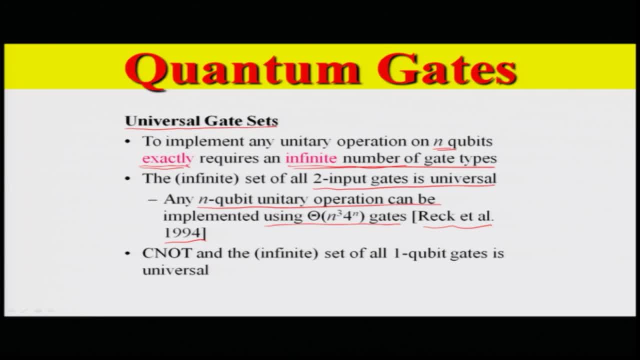 of taken from some work which was done back in 1994 by Reketal, where they were able to show how many operations, unitary cases and orders of the gates that are required for this. So it turns out, as I mentioned, that it is not quite possible to come up with finite 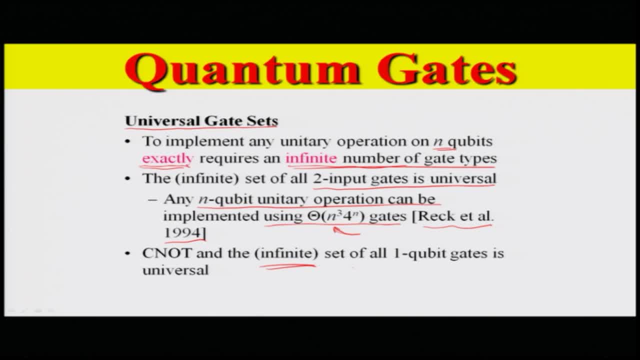 number in these cases. and so C naught and the infinite set of one qubit gates is universal. So C naught is two qubit universal gate, and. But then there are the other infinite set of all one qubit gates that are universal. 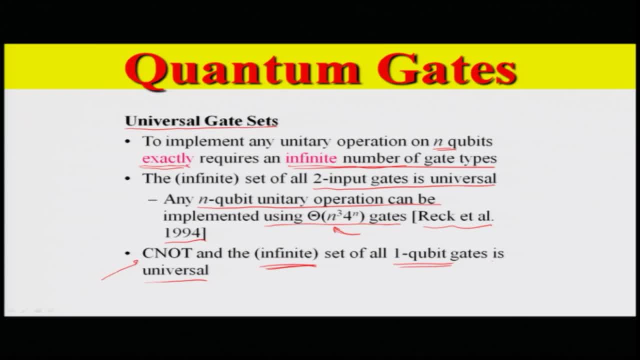 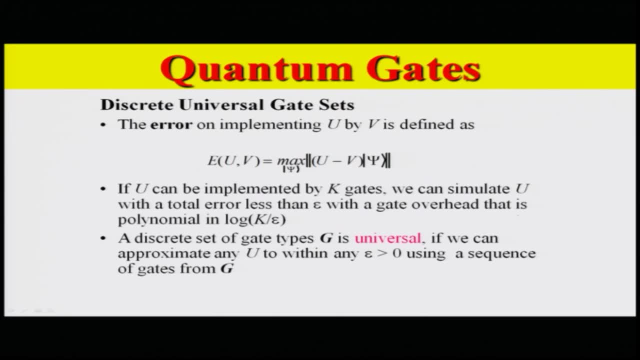 So that is why it is difficult to keep on defining finite set of gates which will make it universal in this kind of an approach. So in order to have discrete universal gate sets, the error on implementing, say, particular unitary operator U by a set of unitary gates. 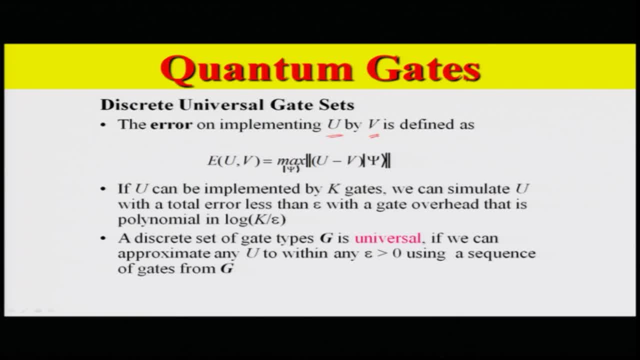 can be defined in this kind of a functional form And if we can have U gates that can be implemented by K gates, then we can simulate that many unitary gates with a total error less than eta with a gate overhead that is polynomial in the order which is log K over. 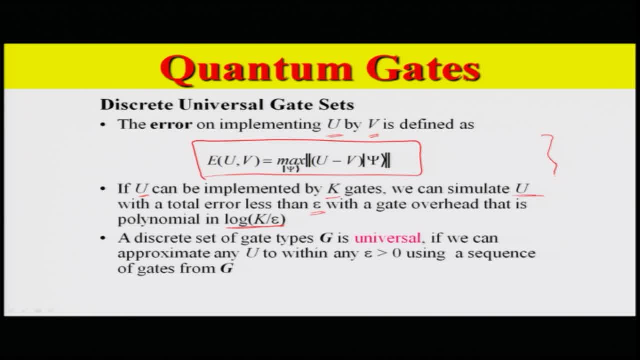 E. Now these kinds of work with their proofs are parts of the unitary gates, So the unitary of theoretical approaches to quantum computing, which is beyond the scope, to some extent, of this course we came up to here because we wanted to talk about the universality of certain. 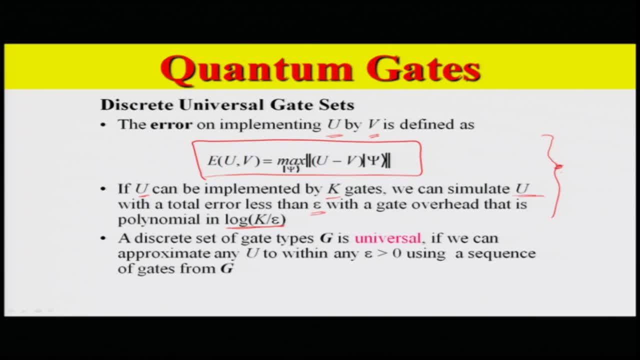 gates, the number of gates are necessary, the closed set and all those which are sort of important in implementation purposes also. However, to be able to get into the exact nature of how many or how to get to these combinations would become difficult. So what we will do is we will take it up to a point. 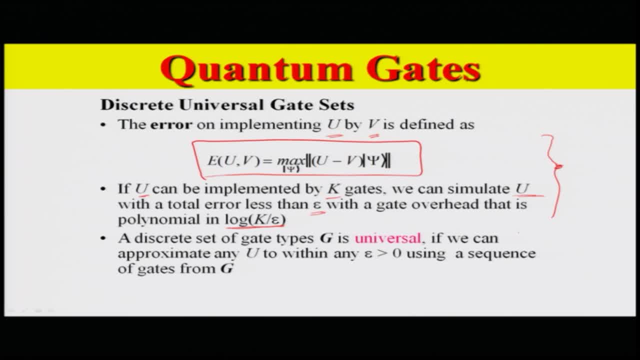 where we have discussed as of now and we will just come to note that a discrete set of gate types G is universal. if this is a statement that we will keep, which is, a discrete set of gate types G is universal. if we can approximate any U or the unitary gate to within an error. 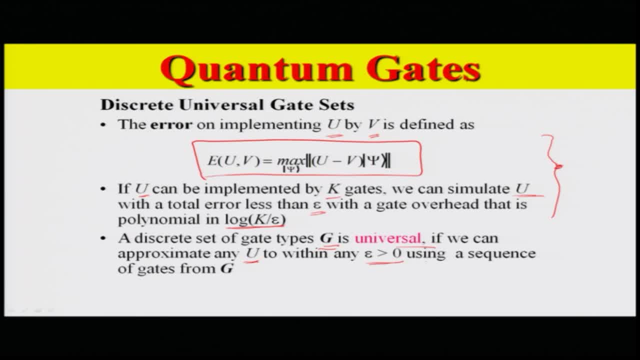 which is eta slightly, not too far away from 0, using a sequence of gates from the discrete gate types of G. So this is sort of a process which is utilized to ensure that, among the infinite sets that are possible, The finite number of discrete sets are often used to within certain level. 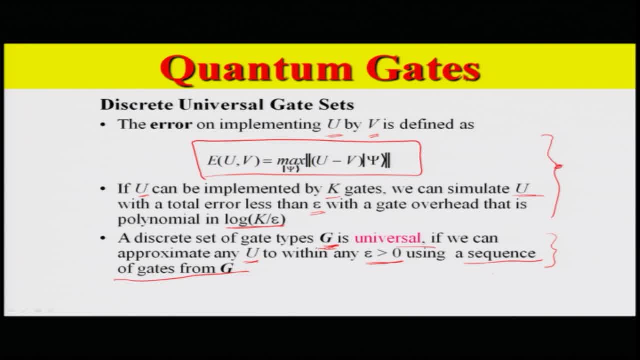 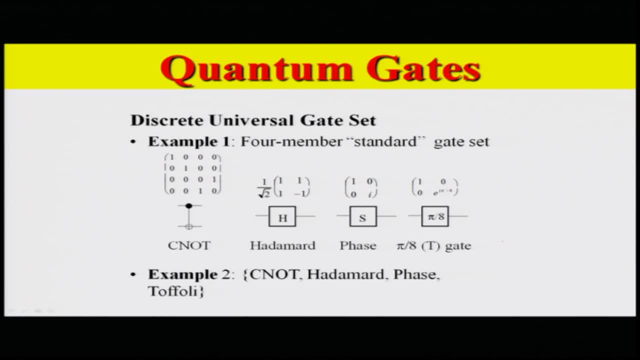 of precision So that the sequence of gates can be utilized with more efficiency. So here is an example of this particular approach. So finally, here is an example of this particular approach of discrete universal gates set. So, for example, four member standard gate set in our 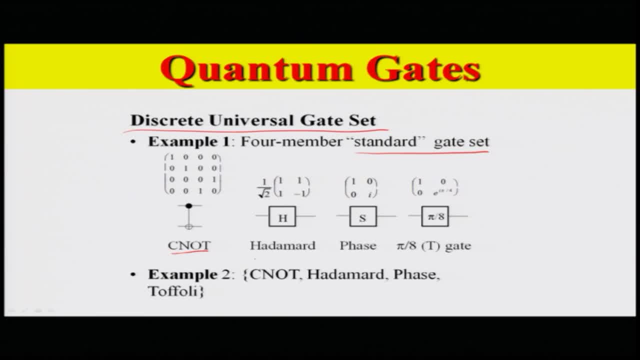 particular approach, as we have been discussing are the CNOT gate, the Hadamard gate, the phase gate and, let us say, the rotation- say here it is a pi over 8 gate- and all of these are the discrete universal gate set that can be used as standard ones. Similarly, there. 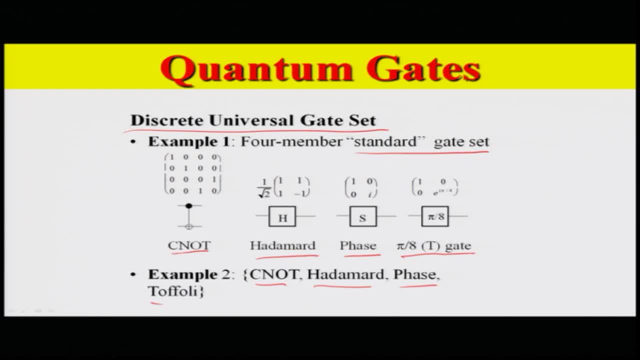 are these CNOT, Hadamard, phase and Toffoli, which can be another set of four gate sets, which are discrete universal gate sets that can be utilized. So with this we just wanted to give you the idea of the different kinds of gates that. 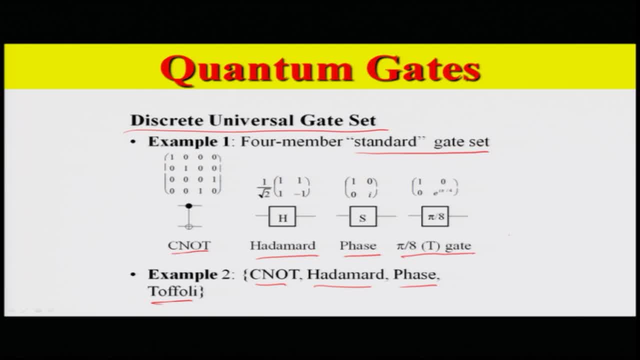 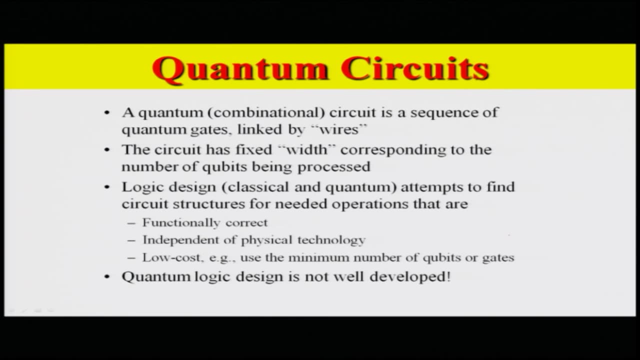 are implementable even with the simple linear optical approaches for quantum computing purposes, and I think we are now ready to look at certain circuits by using this approach. So the quantum circuits are important aspects that are necessary For the overall implementation of the processes and, as far as definition goes, these circuits 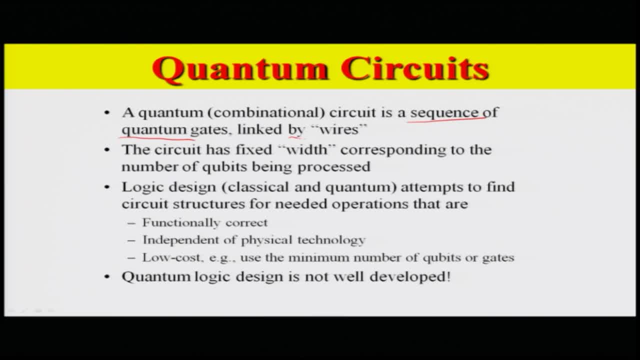 are a sequence of quantum gates linked by wires. They are being put together in such a way that they can implement the processes that we are interested in. The circuit has fixed width corresponding to the number of qubits which are being processed. It is based 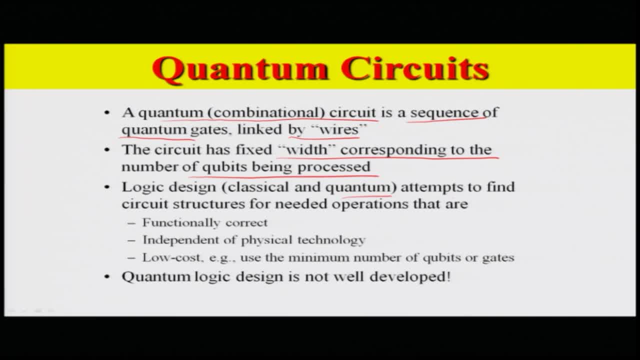 on circuit design, both classical and quantum, which attempts to find the circuit structures for needed operation that are functionally correct, independent of physical technology and obviously for implementation purposes they can require further aspects of low cost or the use of minimum number of qubits or gates. 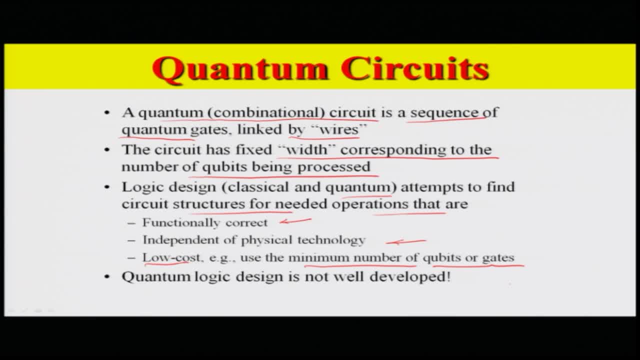 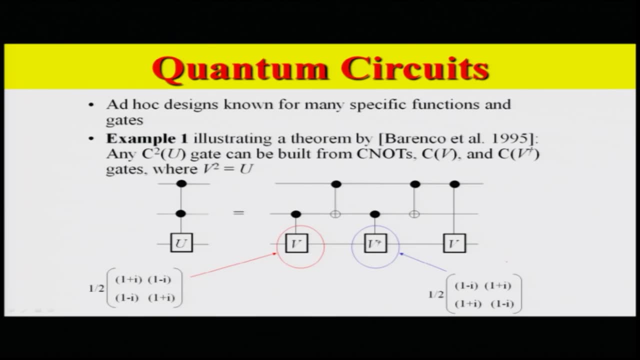 Now, unfortunately, this is an area where a lot more development is presently necessary, As the quantum logic design is still not extremely well developed. There are quite a few ad hoc designs that are known for many specific functions and gates, So here is an example taken from: 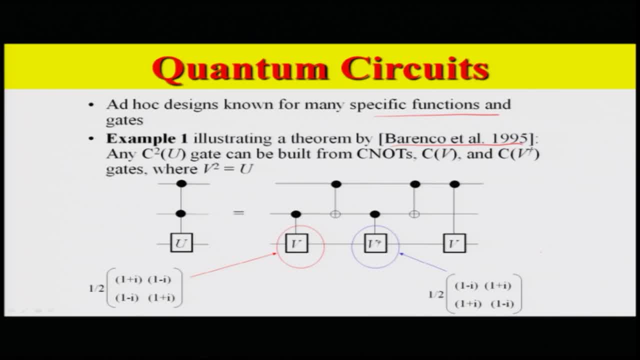 some work done back in 1995, where a Toffoli gate can be built from C knots, control knot gates, Where the a particular gate's implementation twice was essentially a unitary gate. So here is, for example, a particular approach which has been shown to implement certain 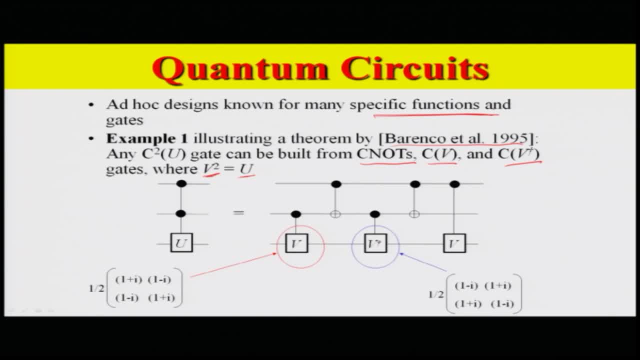 specific functions and this is how some of these wires and circuitry can be written. So the final unitary operation is essentially equivalent to the application of gates corresponding which turn out to be in this particular order. So for certain specific functions it is possible. 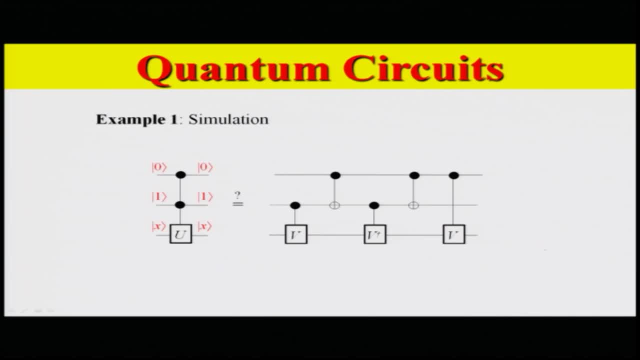 to write them out, as has been done here. it is sometimes important to go through with them. So here, if we know how this is going to go through, then here is an example of what happens when we put in, say, the three qubits in such a particular circuit diagram. 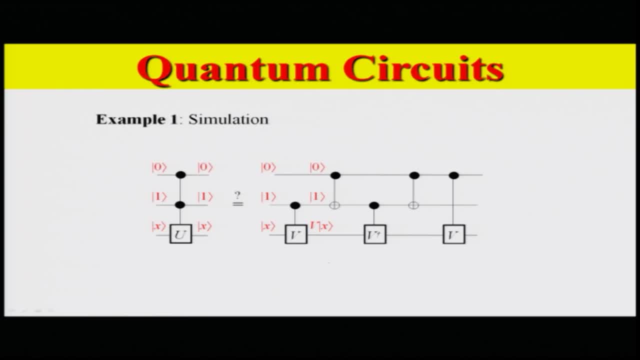 So once we put in these three bits through this equivalent circuits, which is an unitary operation, what we will find is that they will undergo changes as per the sets which have been provided and finally, we will end up producing a unitary operation which results. 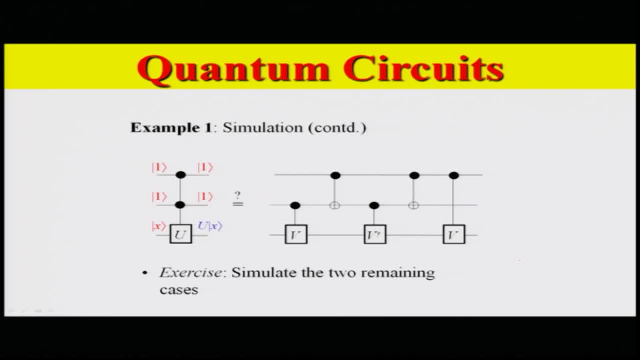 in giving rise to the same result, So it can produce different conditions depending on what the inputs are. So, if you have noticed, my control bit has changed between the last case that we looked at, where my initial bit was 0, now we have changed it to 1 and we can immediately see the control not part being 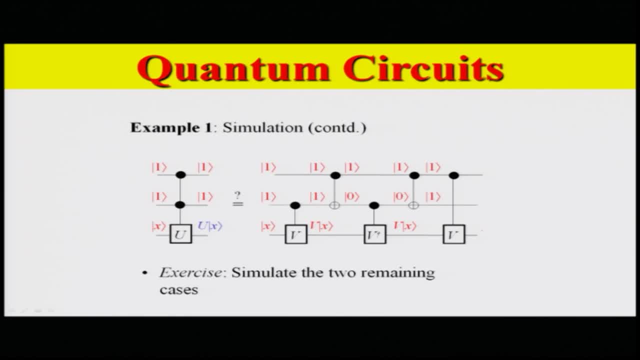 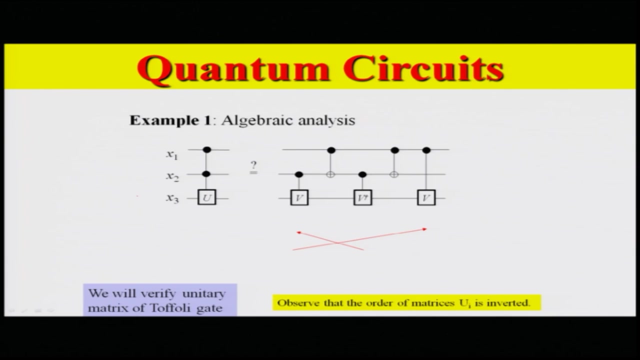 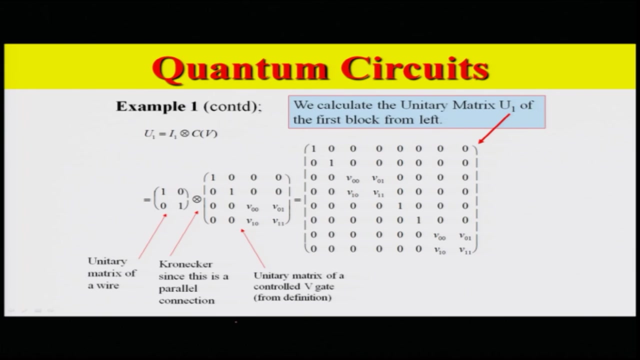 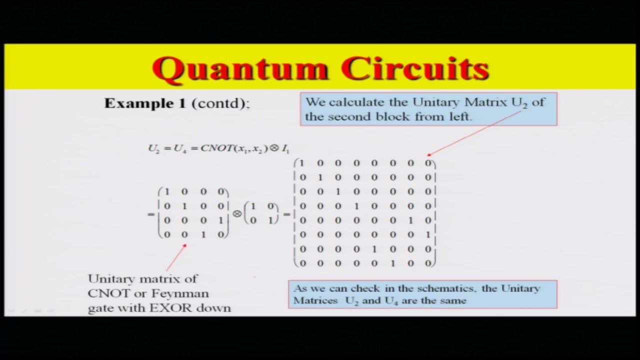 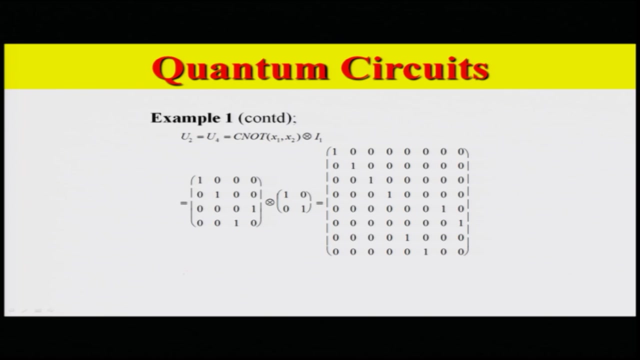 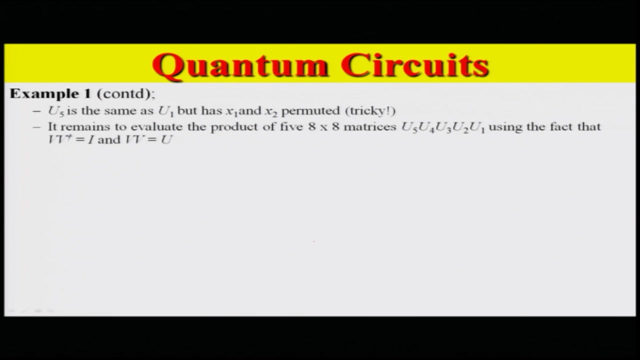 operated on the different points and can see the resultant Situated, and that is why it is a tricky situation. it is not really remaining the exactly same, as we say, and it is important to evaluate the product of all of them, one after the other. 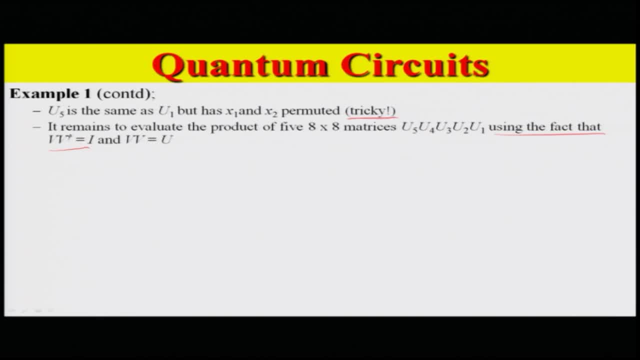 using the fact that we now have them going as identity matrix and applying them one after the other is going to be unitary matrix. So this can be looked at in this entire process. very sparse matrices. all it matters are those little points where they are going to interact. 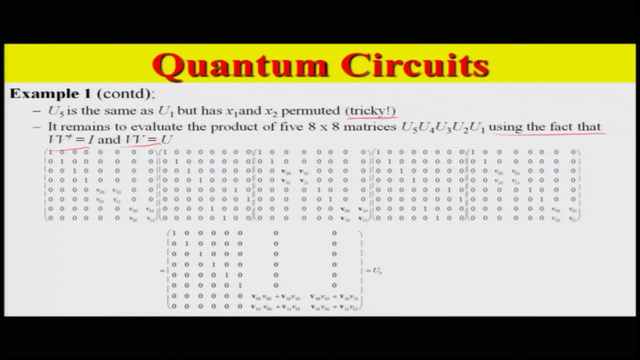 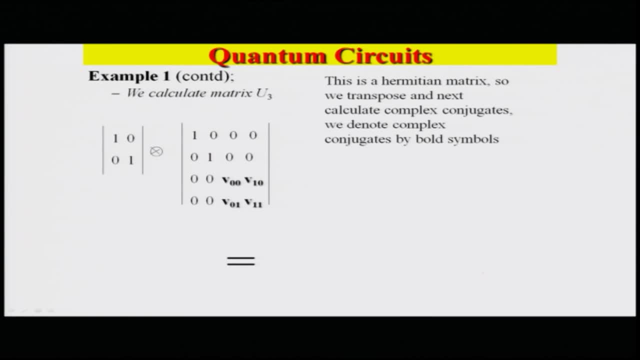 and finally we end up producing the particular sets where they are going to undergo the changes to give rise to the final result. We can similarly calculate the different U 3 matrices that will be necessary for this and which is a Hermitian matrix, So we can transport and 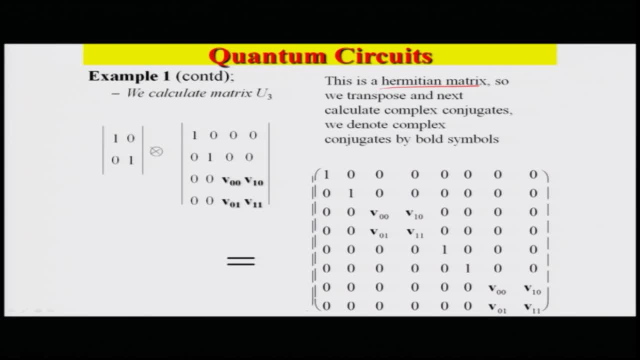 next calculate the complex conjugate. we can denote the complex conjugates by the bold symbols. that is what is being done here, And in all these cases, these different unitary matrices that we have been using are essentially one after the other, and that is why they have. 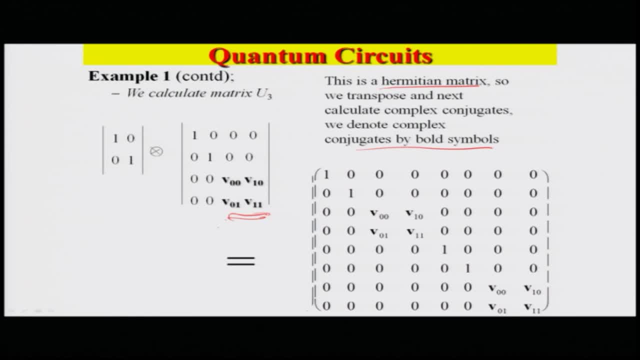 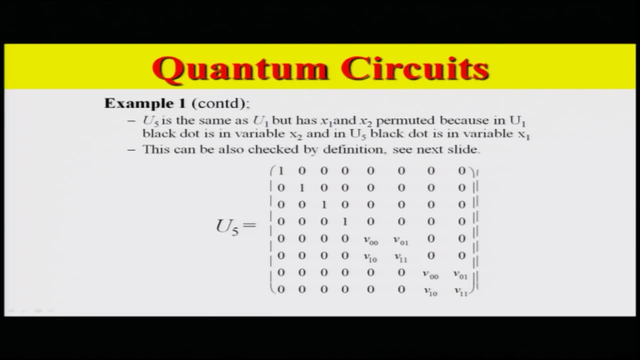 been labeled as 1, 2, 3 in the subscript and that is how they have been shown here. So our fifth iteration, once we go one after the other, is going to be similar to U 1, but has the x 1 and x 2 permitted, because U 1 is in that other fashion where we had a black. 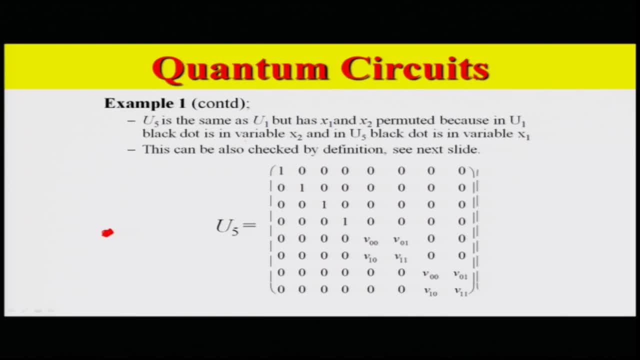 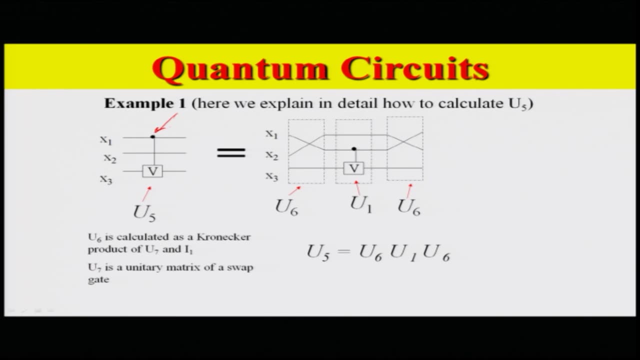 dot- closed dot- in the variable x 2 and the other one is in the variable in the x 1.. So this can be also checked in the Definition which is here. so we had this situation here which was getting connected, and so this. 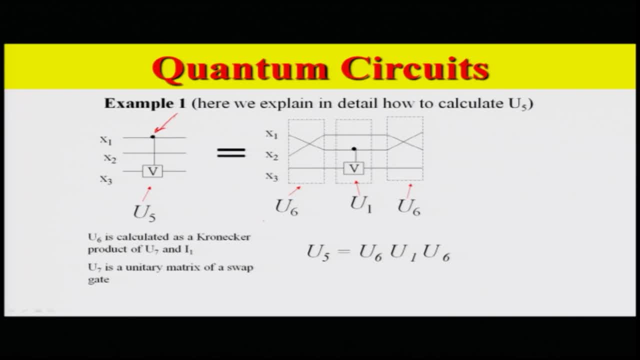 is calculated by using this principle which we started off, and so at every point, whenever we are doing the simulation, so the calculation, this is how they are evolving and we are looking at the final result. The next step would be a unitary matrix of a swap gate, and we can. 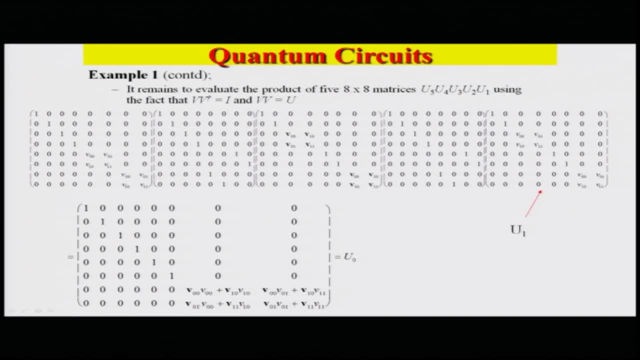 use the five different products of the five, eight by eight matrices which go all the way from one to five, using the fact again that their product is an identity matrix- the V and the V dagger, whereas the their simple product is going to give rise to the 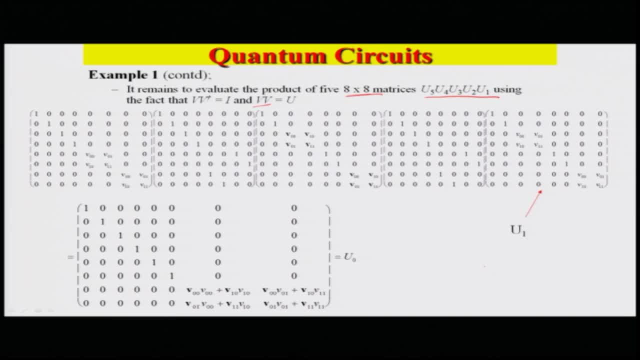 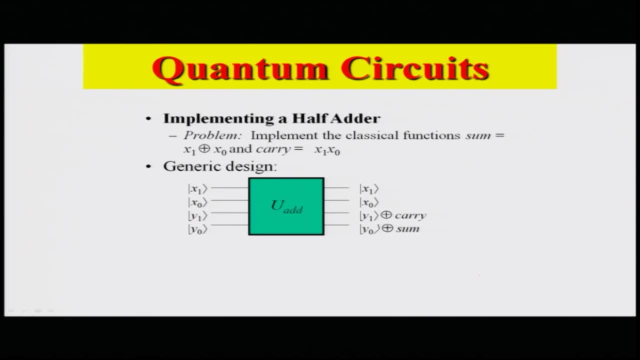 unitary operation, And we can go ahead and find the solution here. So in many ways, this whole process can be brought together by implementing each and every step in the matrix way, as I we just pointed out. The implementing of the half adder, on the other hand, would mean that we have to implement a classical function which 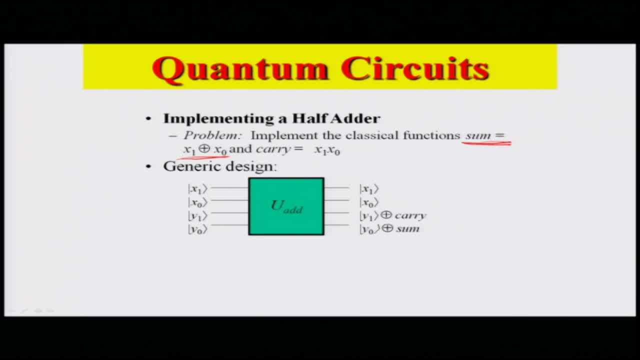 is a sum of the two modulo's and then carry on the product of the X 1 and X 2, X 1 and X 0 at the same time. So these are our inputs and input qubits and these are our outputs, where we have the carry and the sum going in the 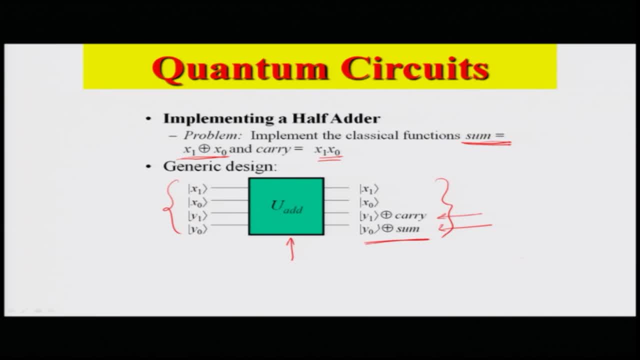 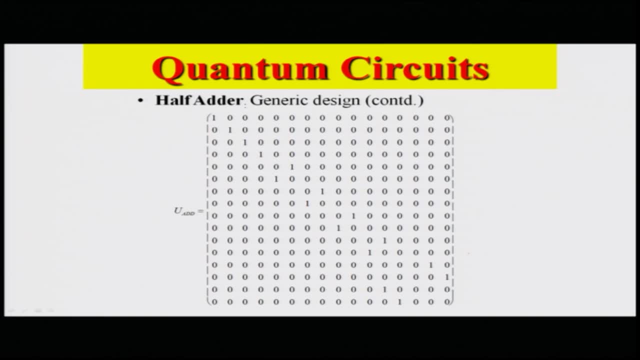 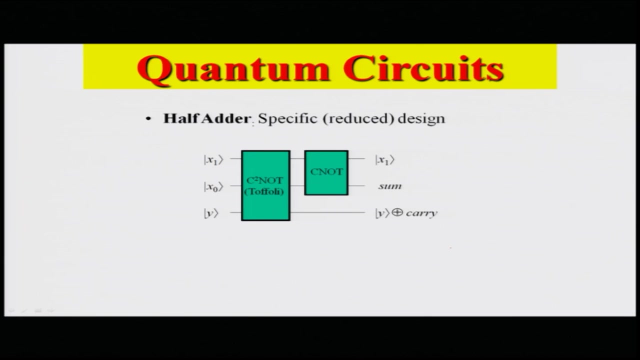 last two bit, and this is the half adder that we are looking at. So a generic design can therefore be implemented by designing a matrix of this kind, where all these elements would then be going through the different principles, as we have been discussing as of now, And the specific reduced design would then be comprised. 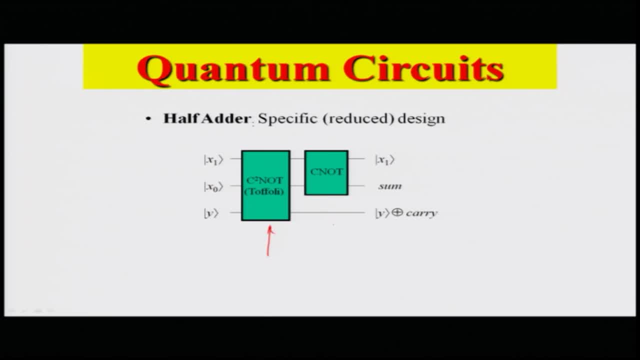 of a Stifoli, which is a control control naught, and a C naught to finally give rise to the carry forward one, as well as the sum of the two which we have used here on the control, which is our X 1.. 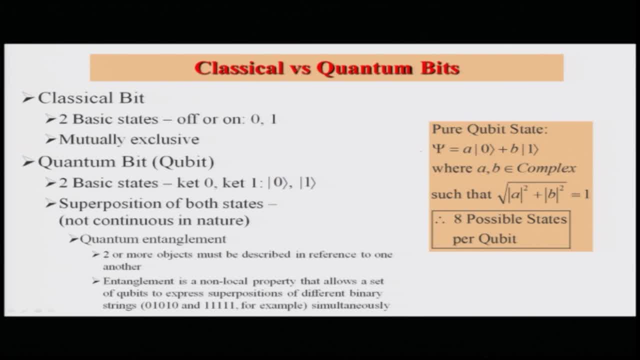 So there are specific differences that we have seen in terms of the classical versus the quantum bits, as we discussed here. The classical bits were very basic in terms of off and on or just the specific numbers, whereas and they were mutually exclusive. However, in our particular case, as we always know, the qubit has many, many states which are: 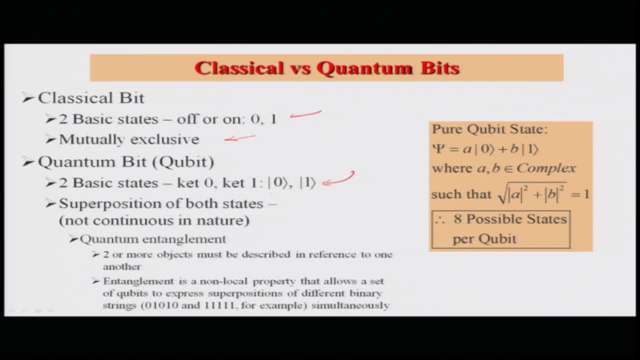 a resultant of the initial ket 0 and 1 and they result in the superposition of states which are non-continuous in nature and it gives rise to entanglement and they can be described in reference to one another, which are non-local properties, which allows a set. 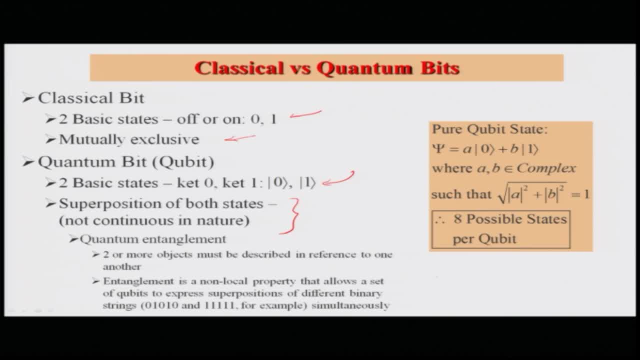 of qubits, to be expressed as superposition of different binary strings. In terms of the qubit state being pure, what we have defined is that they are non-local. they are superposition of their individual states, with their complex coefficients, such that the square of the mod of those coefficients would give rise to be equal to 1,. sum of this: 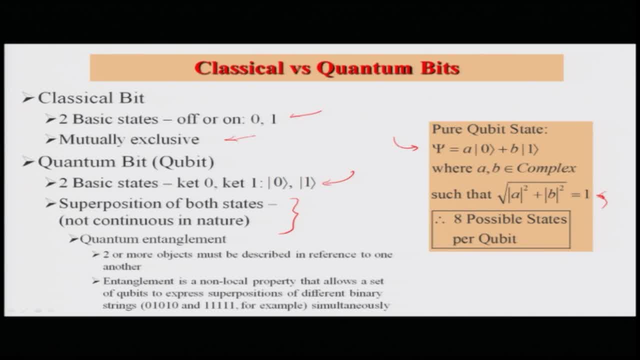 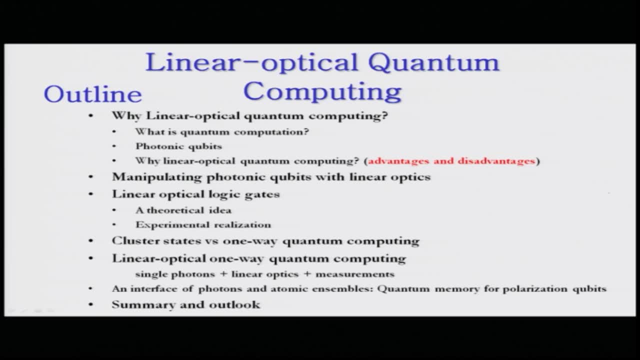 mods of the square, which means that they are normalized and, as such, there would be eight possible states per qubit. With this background, let us revisit the process or the principle that we are looking for. This is the linear optical quantum computing process where we have been essentially going. 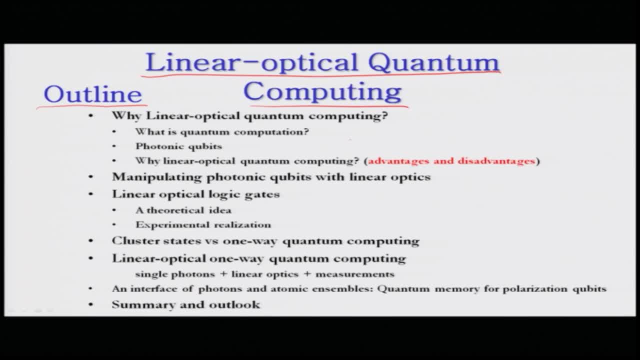 over the details of these quantum computing aspects with respect to approaches of linear optical designs. These are in some sense our photonic qubits, which are our photons, either in different polarization states or as different momentum states. They have their own advantages and disadvantages. 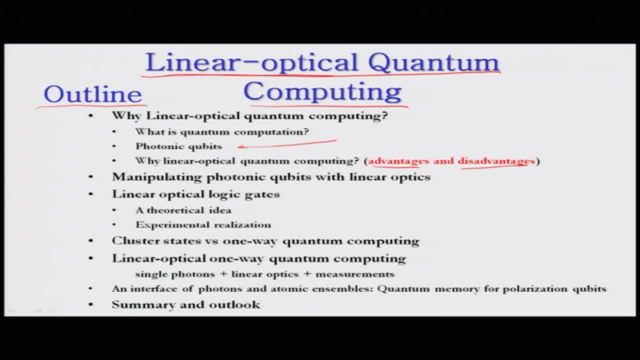 As we have been discussing, there are many other ways of using the optical principles into quantum computing, but those are separate entities. As of now, we are just looking at this particular approach. We could also take advantage of photonic qubits with linear optics. 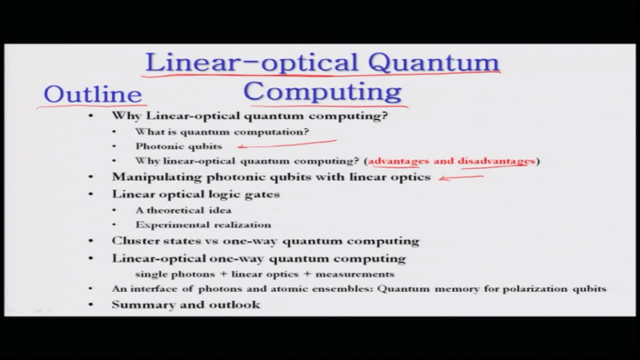 in this particular process. The linear optical logic gates initially started off with the theoretical idea, but has been put into experimental realizations by using beam splitters, polarizing and linear optical logic gates. The linear optical logic gates initially started off with the theoretical idea, but has been put into experimental realizations by using beam splitters. 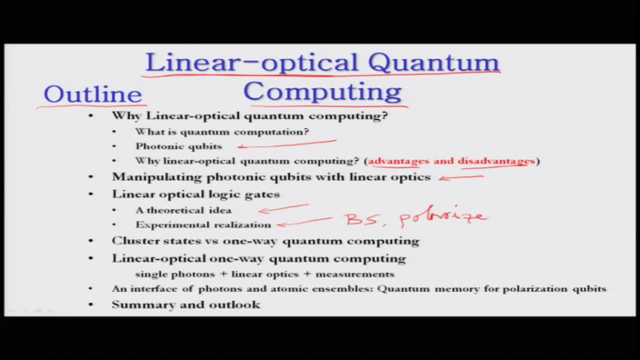 polarizers and wave plaits. There are also approaches which are clusters versus one way, quantum computing. I do not know if you will be getting into these areas because demonstration aspects of these are still very sparse, but these are different ideas. Once again, linear optical, one way. 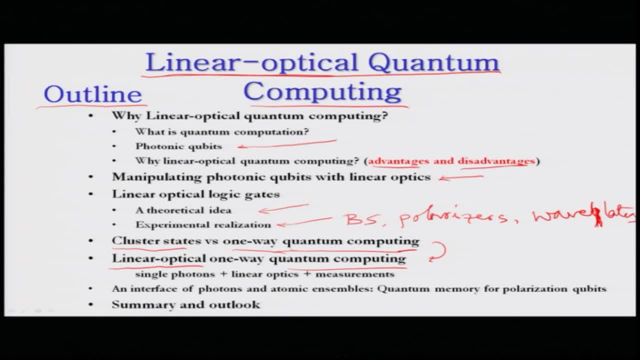 quantum computing has been developed as a result of this understanding, which uses single photons, linear optics, as well as their measurements And interface of photons and atomic ensembles have been used for quantum memory, for polarization of qubits, and we will finally look at their 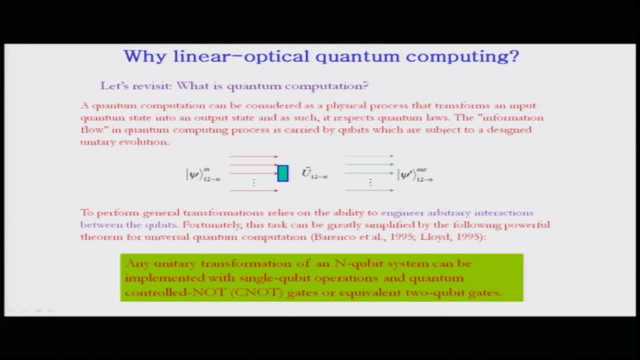 summary and outlook as we go along in this direction, So revisiting this whole principle. we can understand as to why we would like to have this principle of optics coming into this picture of quantum computing and that to linear, and because that has the advantage where the information flow in the quantum computing. 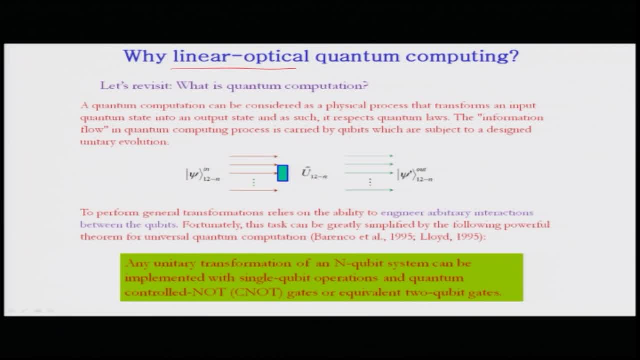 process can be carried on by the qubits, which are subjects to design unitary revolution, which are being carried out in this particular case by optical approaches. So performing general transformation relies on the ability of the optical data, the engineering, arbitrary interactions between the qubits. This task has been greatly simplified. 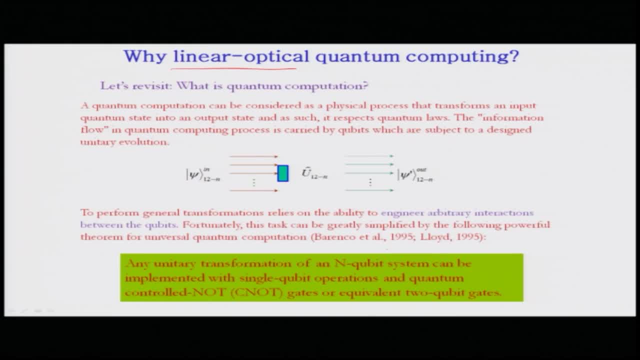 by following the universal quantum computation theorem of Lloyd and others which have been worked on in this area. Any unitary transform of an n-qubit system can be implemented with single qubit operations and quantum control, not gates or equivalent two qubit gates. That is what we discussed. 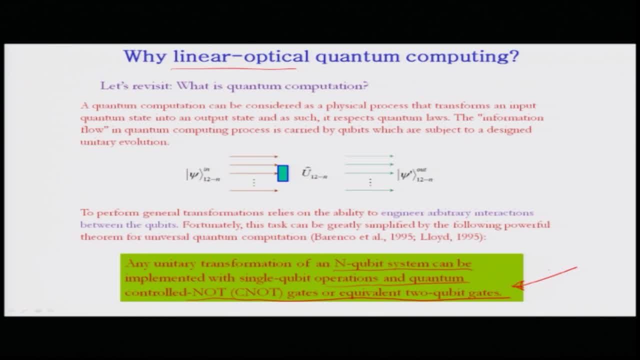 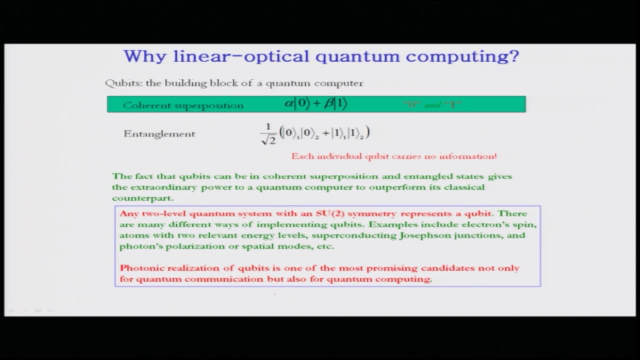 in the beginning part of this lecture, showing that it is important to realize the universality of these processes. Now, the building block of these qubits are our aspects of the superposition, which not only is just a combination, but also it is a coherent process. 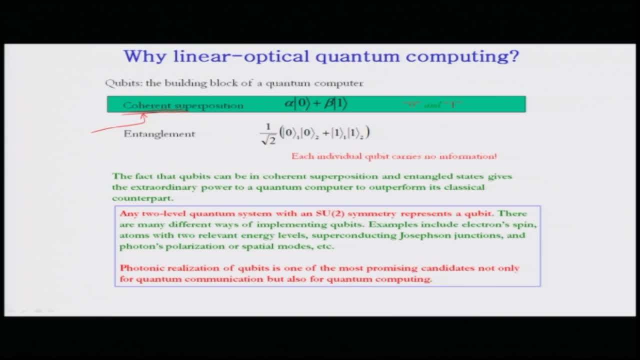 Coherent superposition such that the coefficients can be complex, although their mod squares always add up to be equal to 1. They can also add together in terms of entanglement in such a way such that the individual qubit carries no information at all, but the composite together. 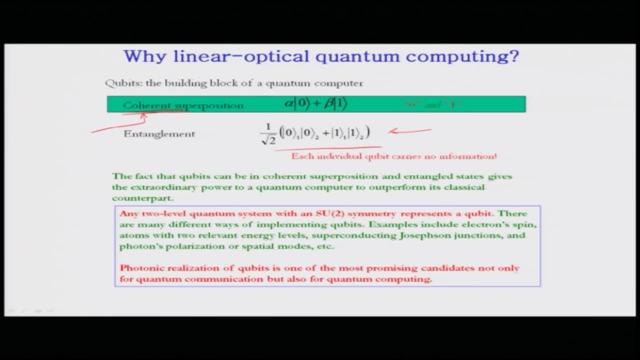 carries all the information. The fact that the qubits can be in coherent superposition and The fact that the qubits can be in coherent superposition and entangled states gives the extraordinary power to a quantum computer. That is what we know and that outperforms. 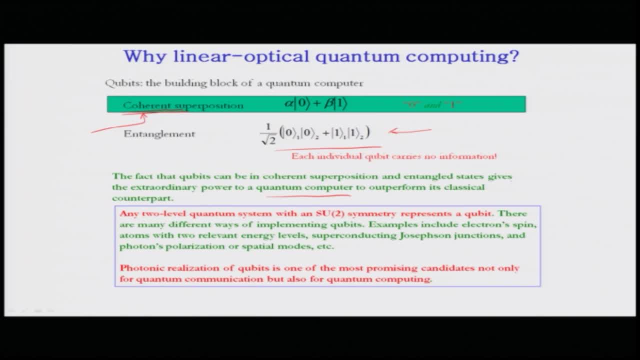 its classical counterpart. So whenever we are using any implementation approaches, we have to see that this particular approach or this particular advantage remains to our particular sense. Now, there are many different ways of looking at this, from mathematical principles as well as several others. There is a subgroup which can be used which has the symmetry of the. 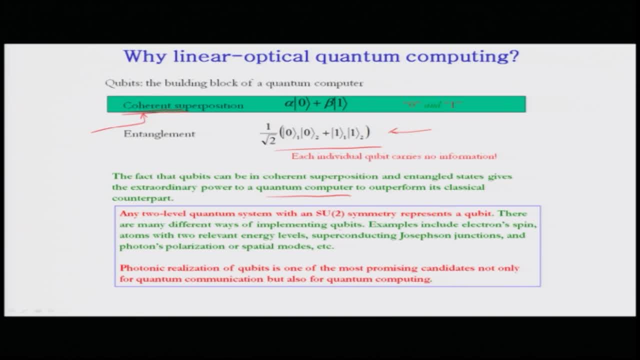 quantum system, For example, a two-level quantum system has SU symmetry and that can represent a qubit. There are many different ways of implementing qubits. For example, we have already talked about electron spins atoms with two relevant energy levels. These 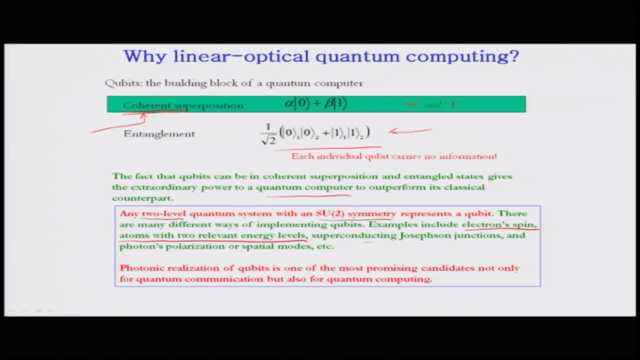 were all talked about in our introductions. We will be talking sometimes later about superconducting quantum functions and photon polarizations or special modes. But the more important part which we are dealing with right now are the photonic realization of the qubits, which is one of the most promising, not only because they are easy or important. 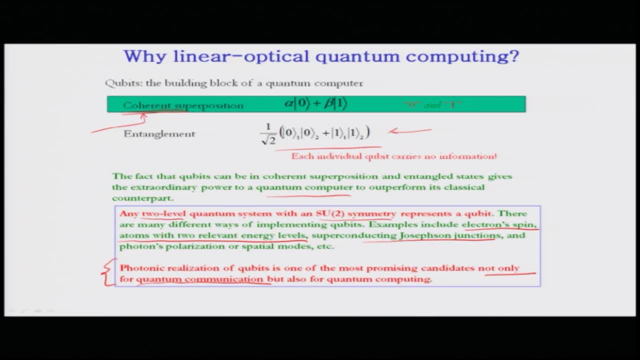 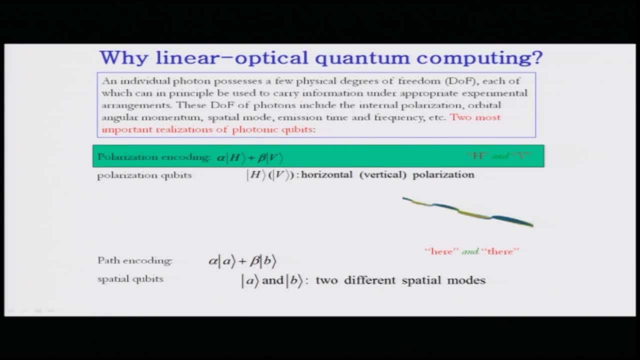 but also because they are the ones which are important for quantum communication purposes, as well as for carrying forward quantum computing to multiple scalable levels. That is what we are after. A QBIT can be used for both horizontal versus vertical polarization. It could also have 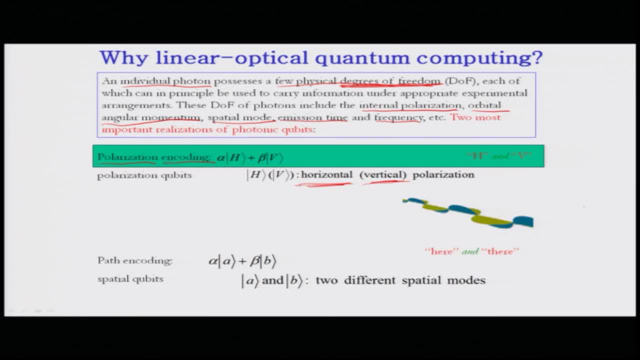 counterclockwise versus clockwise circular polarizations. Either way, it will have the polarization qubits. The path encoding could also involve their presence where they are here and there. that is the momentum approach. have special qubits which are based on the special modes which could be the different. 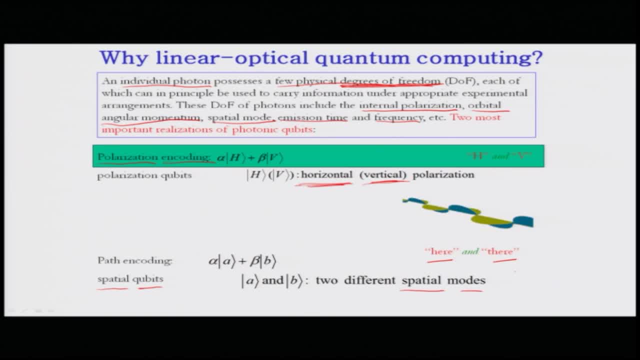 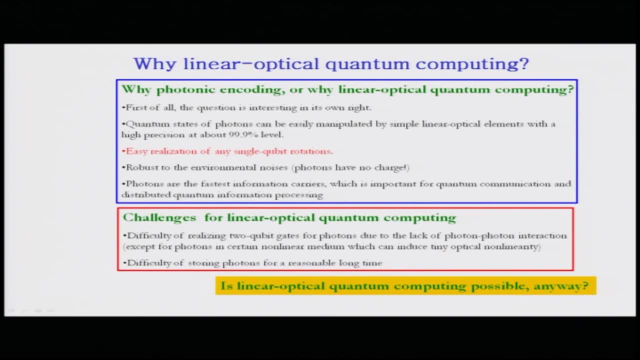 modes of the qubits or the photon that we are looking at Now, the aspects of photon polarization and its encoding has many different ways of looking at it. The quantum states of photons can be easily manipulated by simple linear optical elements, as we have been discussing. It is not only interesting in its own right, but 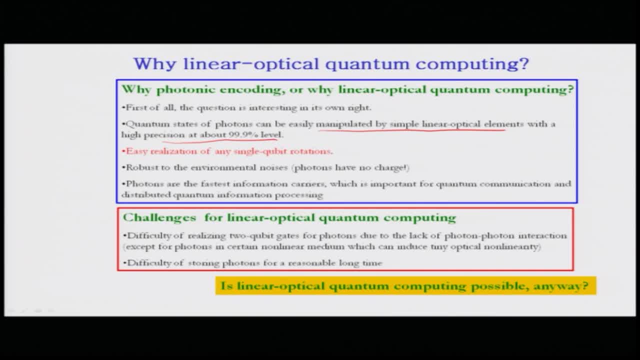 also has this high precision of about 99.9 percent accuracy. It is easily realized with any single qubit rotations. It is robust to environmental noises. Photons have no charge, so they do not interact and create a problem for the other. 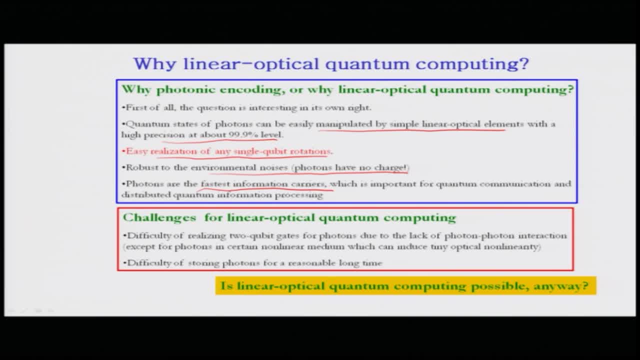 They are also the fastest information carriers, which is important for quantum communication. However, the challenges are also not that simple. Difficulty of realizing two qubit gates for photons is due to the lack of photon-photon interaction. The very process which makes it robust also makes it difficult to scale it up. So there are many newer approaches. 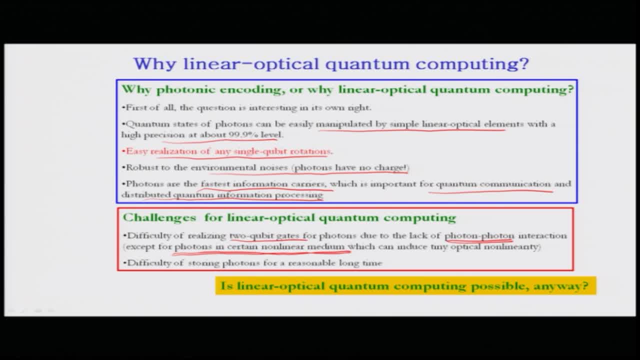 which rely on utilization of non-linear media- And we will get into that also- And the other very important part is the storing of these photons for a reasonable long time for this particular approach. So there has always been this question as to whether it is possible to scale up or do other things into the future. 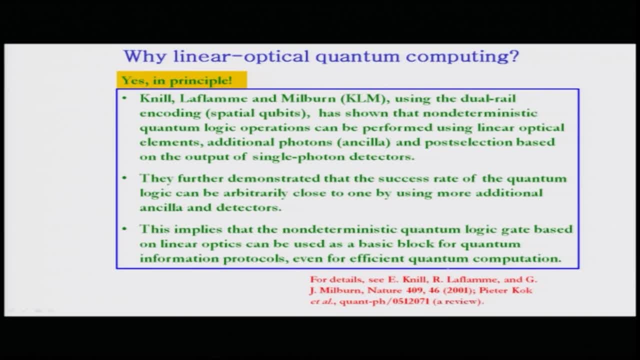 But as demonstration purposes. this has also remained as a very important approach And in principle. a lot of work happened in the early 20th century. The first development was done in the early 2000, where they have managed to show that. 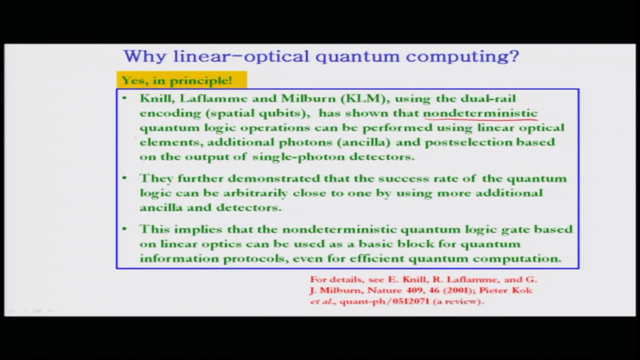 it is possible to show, non-deterministic quantum logic operations can be performed using linear optical elements where, in addition, ancilla photons, which are additional photons which are not participating in the actual process of the computation, are going to give the strength to this process, and the post electron based output of single photon detectors can also. 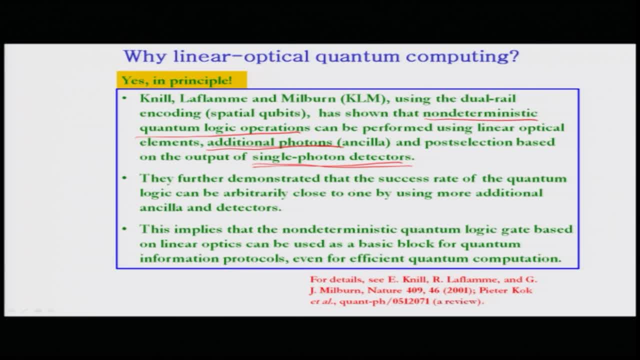 be utilized for further processing and robustness of the process. This group and several others about their time were also able to demonstrate the success rate of quantum logic arbitrarily grows by using additional ancilla and detectors, and this has been a trend in the recent years. lot of developments beyond this has also happened. 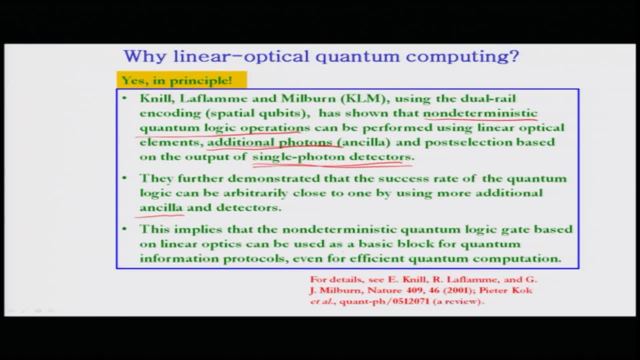 The non deterministic quantum logic gates based on our linear optics can be used as a basic block for quantum information protocols, even for efficient quantum computation. So certain part of the quantum computing development certainly benefits from the optical approaches. There are many different advantages. 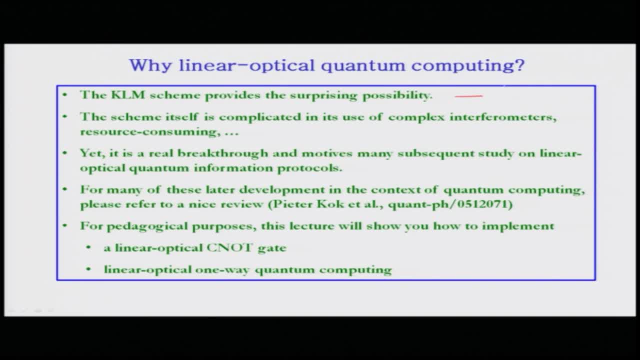 The very important process of the laser cavity itself has been utilized- and while studying about different aspects of laser, we talked about curl lens mode locking for making short pulses, and that in itself has been found to be advantageous for doing certain applications of quantum or demonstrating Grover search, for instance, which we will do in this lecture. 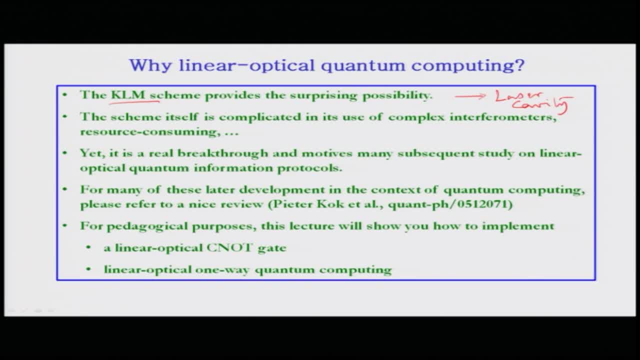 Hopefully within this week. the scheme itself is complicated and in terms of the linear optical approaches because it may use complex interferometers and it is often resource consuming because, being linear, often the number of resources necessary for this process is quite high. However, it is a real breakthrough and motives where many subsequent studies on linear optical. 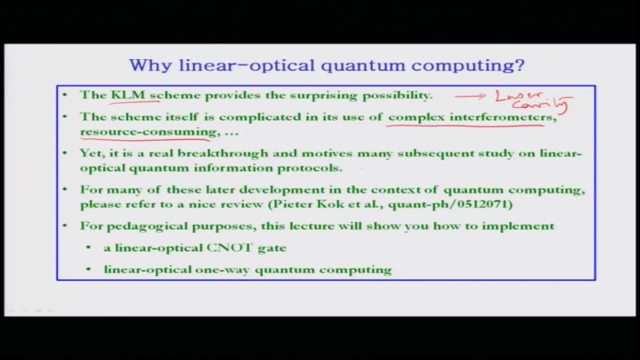 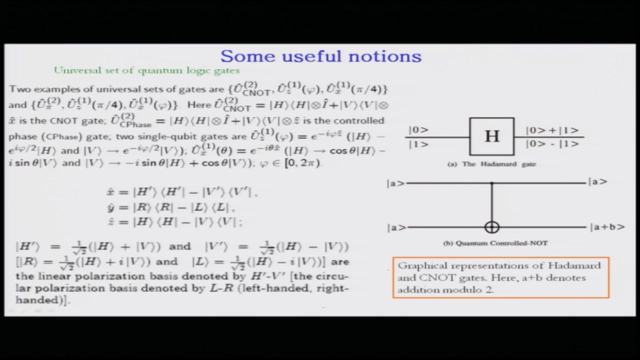 in quantum information protocols have been applied, Thank you. There has been some recent reviews and other work, but what we will do in this particular lecture is to show you how to implement a linear optical CNOT gate. We will demonstrate in some process here. 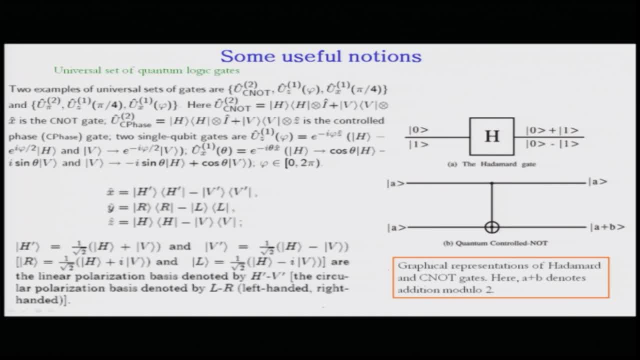 In some sense, this is something which we discussed in the last class, where we set up the universal set. We set up a set of quantum logic gates and then we applied the Hadamard in terms of the beam splitters to be able to show that we were able to combine the input gates into 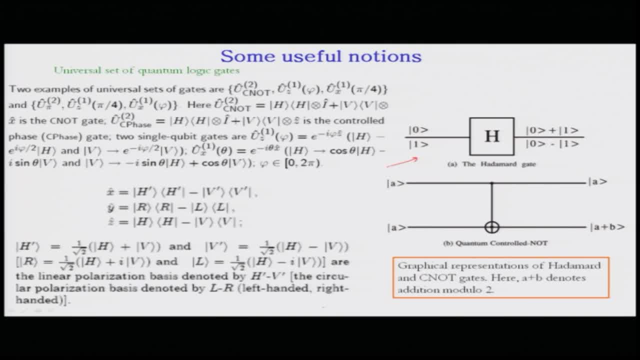 a process where we would be able to use them and similarly, we would be doing the graphical representations of the Hadamard and the CNOT gates and since it is a process where many of this has been already looked into. So let me end today's class because we have already come to a point where we have 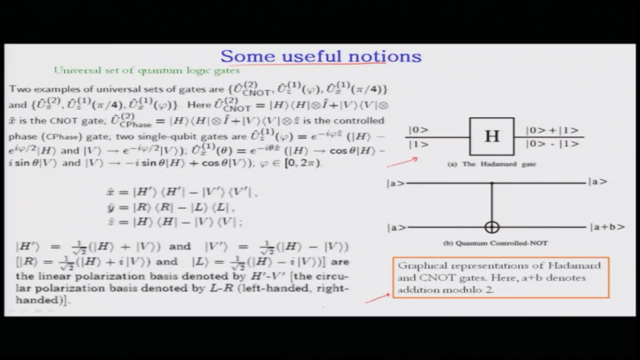 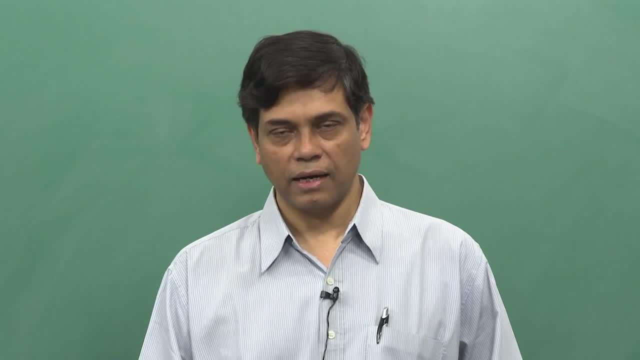 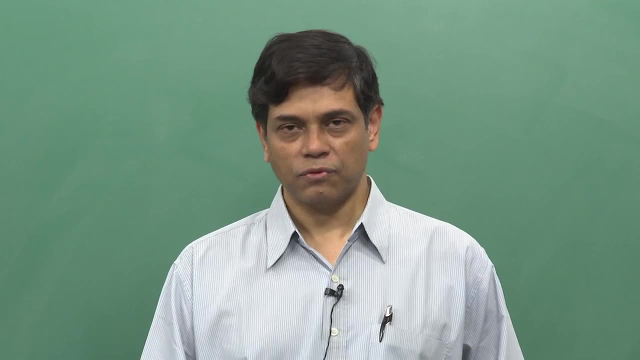 covered most of these aspects before, And so let us close this lecture by mentioning that linear optical approaches to quantum computing and the various gates that have been designed in this process based on the photon properties, seem to be very effective in many ways. 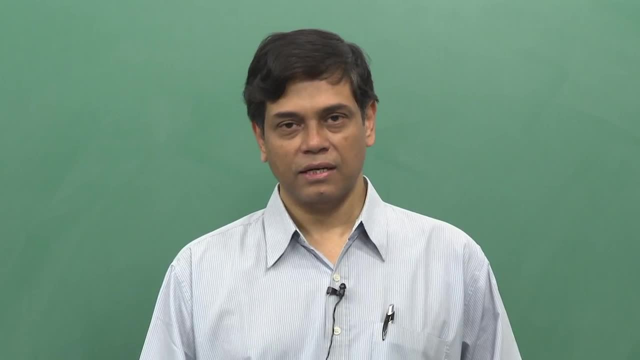 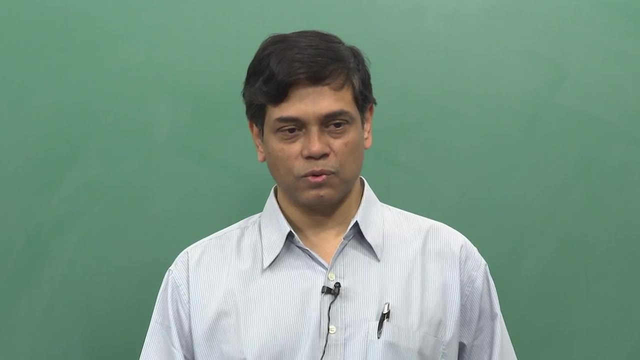 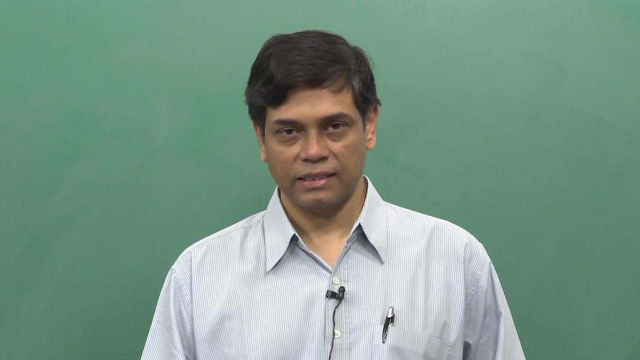 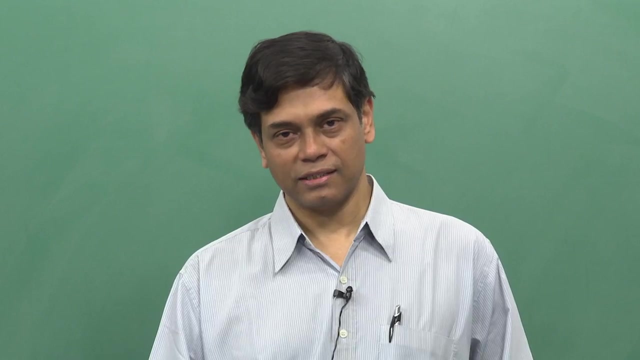 them to benefit and demonstrate quantum information processing. One of the very different approaches to quantum information processing with optics has also come by in terms of using a laser cavity itself to demonstrate Grover's algorithm, which we will do in the next class, and I think you will enjoy that a lot. So with this, let us close today's class and we will see you next week. 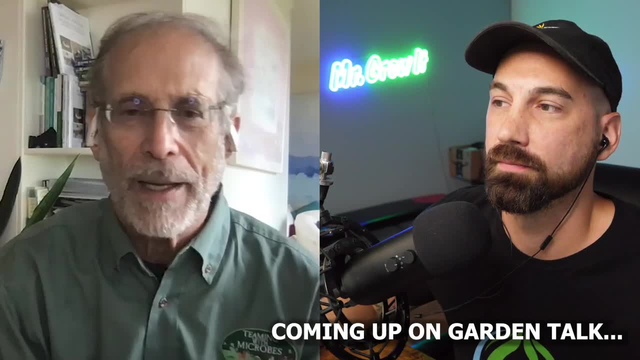 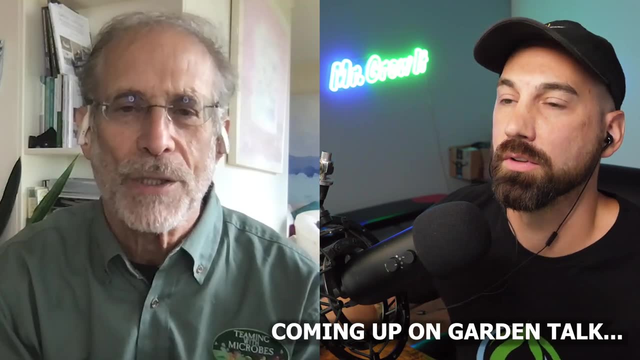 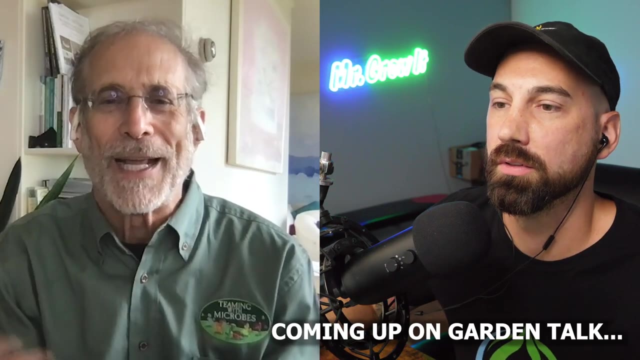 Coming up on Garden Talk. If you're adding algae to the soil, if you're adding rock sand, whatever you're doing to the soil, you can come back and measure it two or three, four weeks later and see whether it's having an impact increasing the biomass, Because if it is, you want to continue to do it.